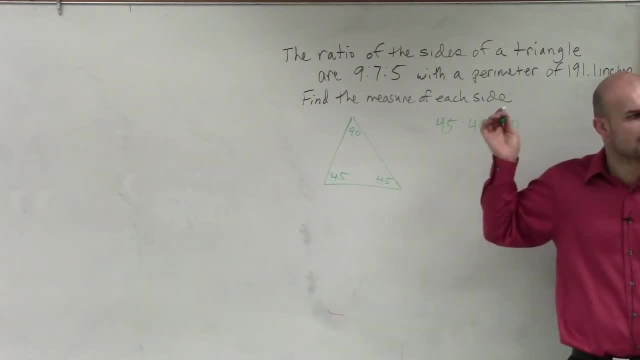 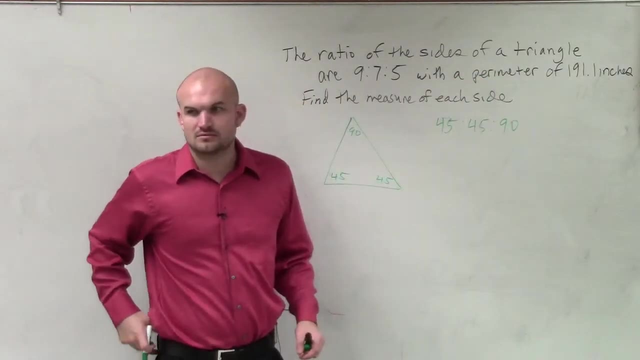 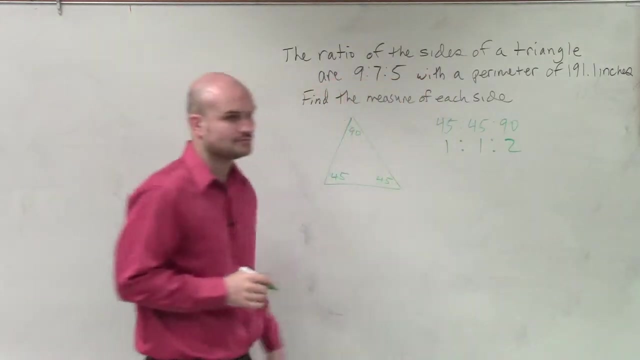 Right, That's how they compare. That's all the sides of the triangle compare to each other. Does everybody agree with that? Okay, But is that simplified? No, You can divide 45 into all of those. So really, the ratio of the sides is 1 to 1 to 2.. Right, And what? 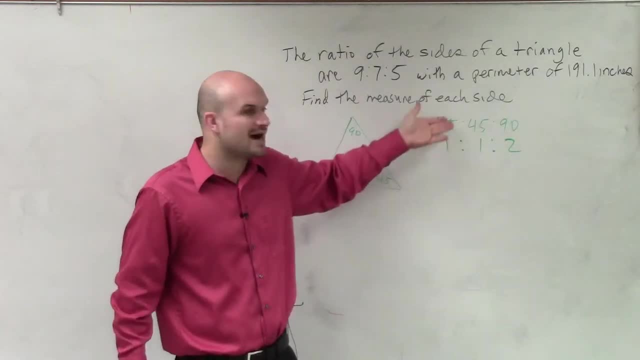 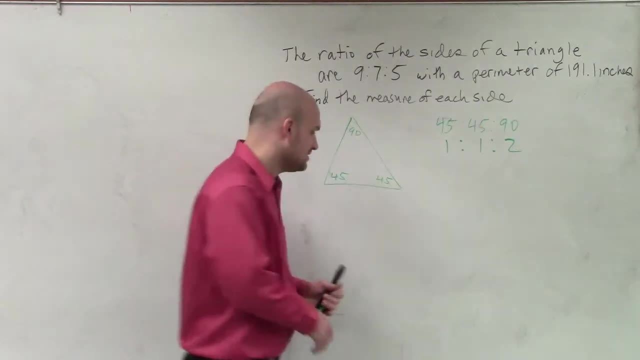 we want to do is we want to be able to determine: well, how do I get from 45, 45 to 90 to 1, 1, 2? So I'm going to divide that by 45. But let's say I took that away and I say: hey, here's. 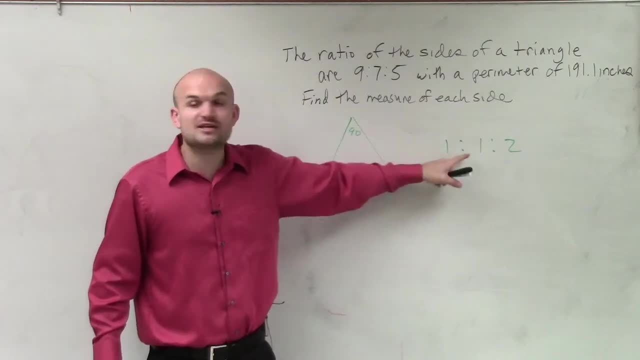 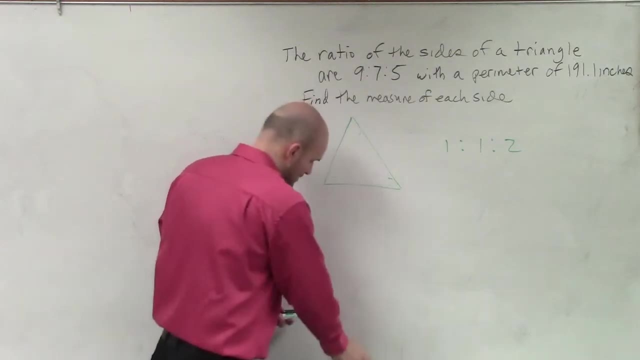 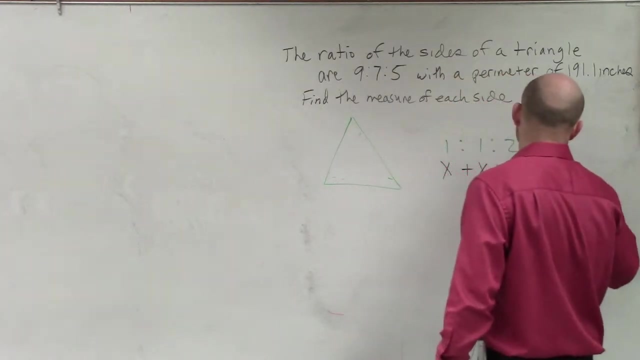 the ratio of the angles. Here's the ratio of the angles. What is actually the real angles of the triangle? Let's say you didn't know they were 90,, 45, and 45. So what we would do is we'd actually have to write an equation: X plus X plus 2X equals 180.. All right, Where? 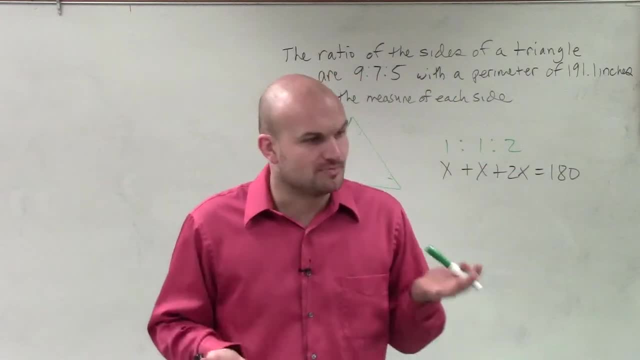 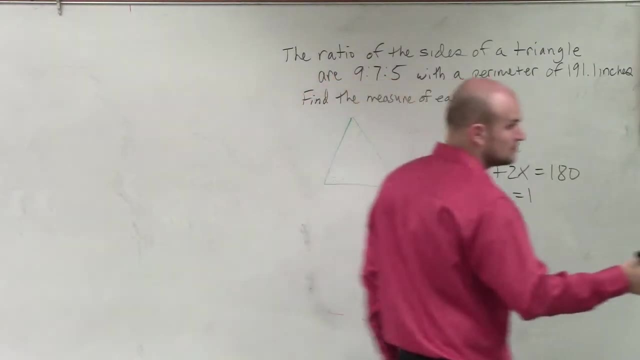 X is what is going to be the factor. So what we're going to do is we're going to divide that by the 16th factor that we multiplied or divided to be able to get our angles. So, therefore, I would solve this, which I'd get 4X equals. Okay, Thank you. Is she supposed? 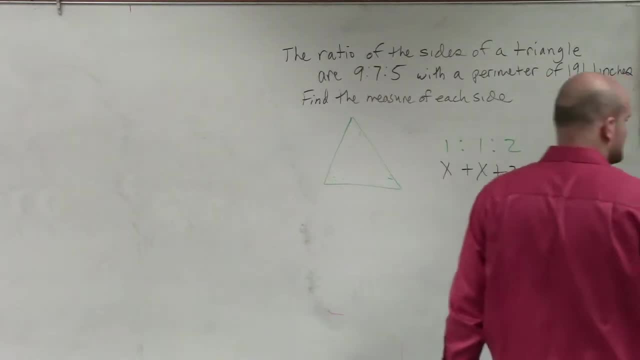 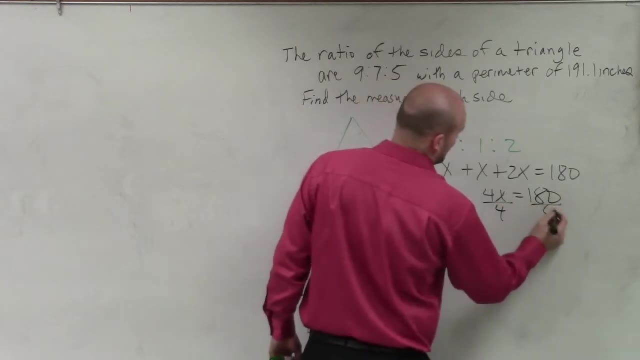 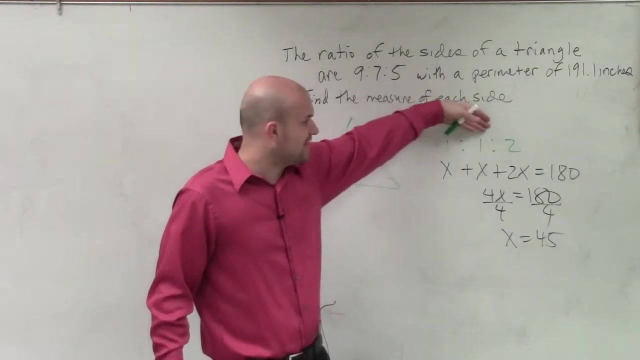 to be in here. Okay, 4X would be 180.. Divide by 4,, divide by 4, X would equal 45. Therefore, you can now see that the new ratio would be 45,, 45,, 90.. 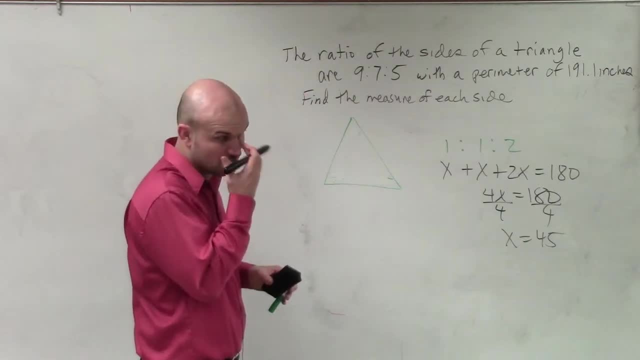 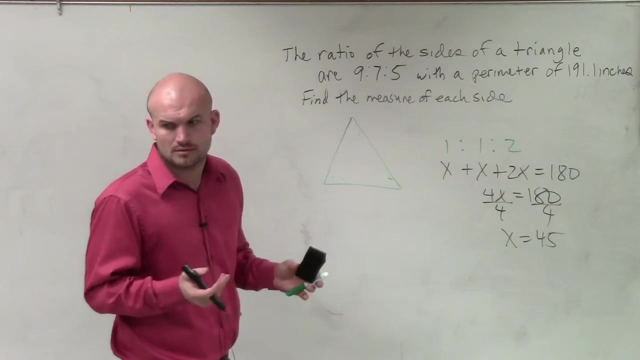 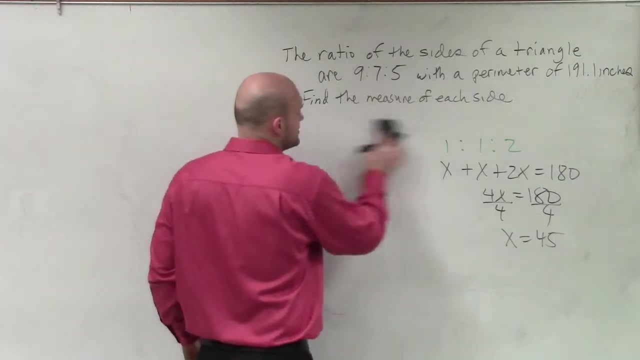 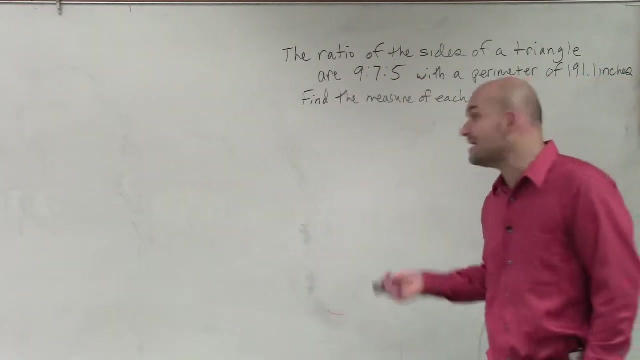 So, ladies and gentlemen, what we're going to be doing is: So let's look at this problem, This problem. they say that your ratio is 9,, 7, and 5.. Well, ladies and gentlemen, we know those are not the actual lengths. 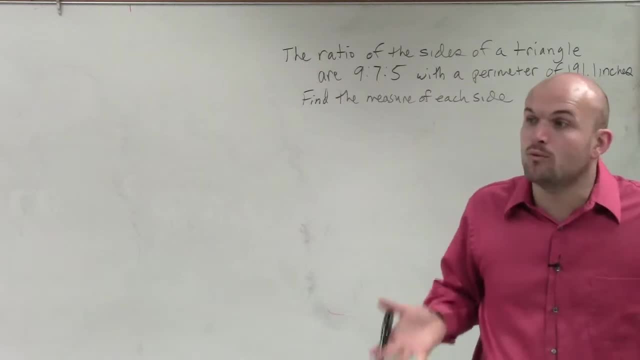 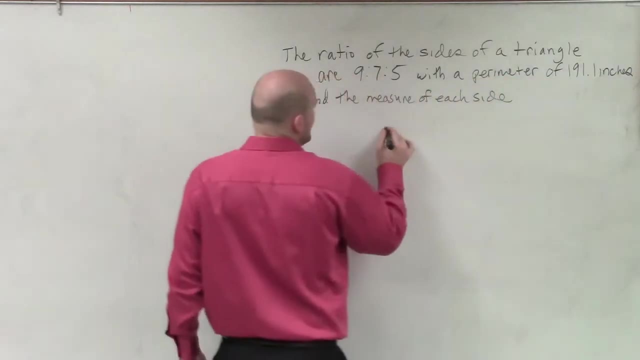 We know those are not the actual lengths. So what we need to do is we need to figure out what did we divide those actual lengths by to get our reduced ratio of 9,, 7, and 5.. So what I need to do is I'm going to write up 9x plus 7x.